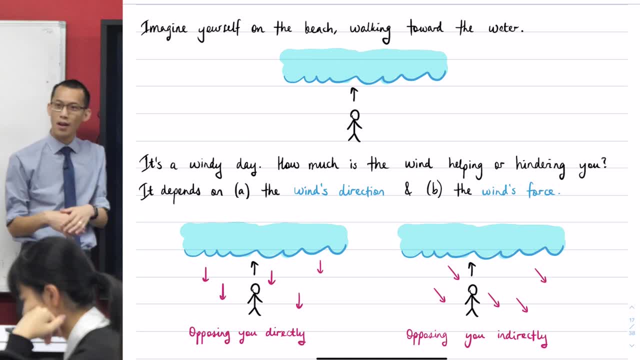 So many different ways that you can think about this. whichever way works for you, I think you need to have some kind of metaphor in your head, whether it's, you know, playing a video game or holding a bucket to rain, or thinking about a windy day on the beach. 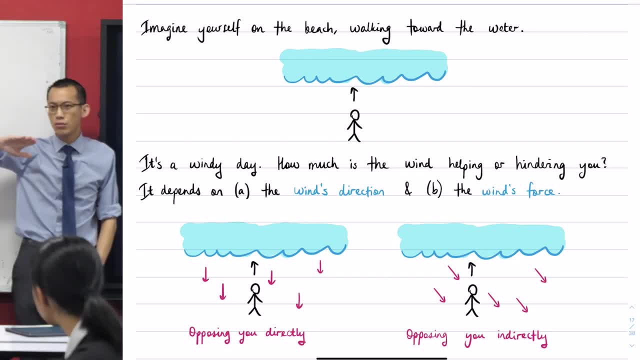 Otherwise you're just crunching numbers, right, And we do not want you to be people who are. We don't want you to be computers. You know computers used to be people, Like that was their job, because we didn't have objects that could do the calculations that we needed to rely on human beings who could compute things right. 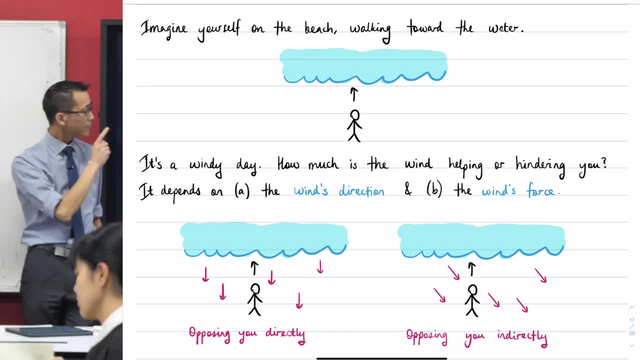 We want to go, We want to pass the computation and think about what does it mean? So imagine yourself on the beach trying to walk toward the water And, importantly, it doesn't matter where in the water you land, You're just trying to get to, you're just trying to get wet, right? 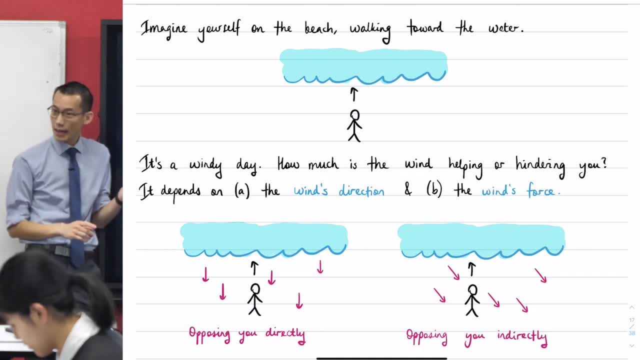 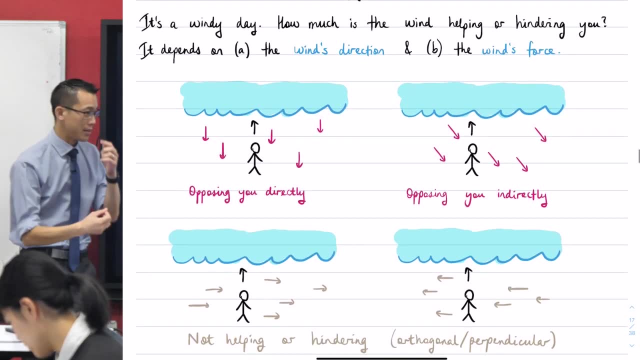 So you're just trying to get out there, okay. Now, if it's a windy day, if it's a windy day, which it often is, at the beach, right. Then the question that the dot product answers is: how much is the wind swirling around you? 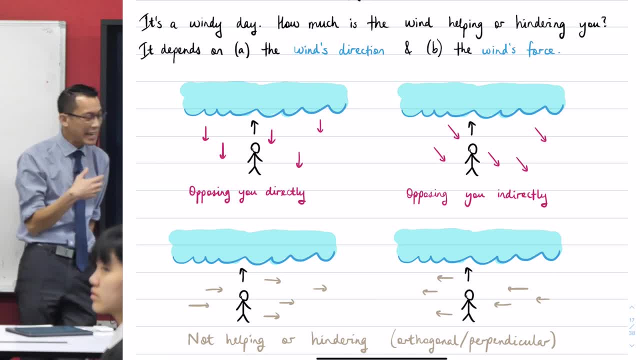 How much is it helping you towards the water Or how much is it hindering you away from your goal- away from the water right Now? it clearly depends on two things, And you can see why this relates to vectors, right. 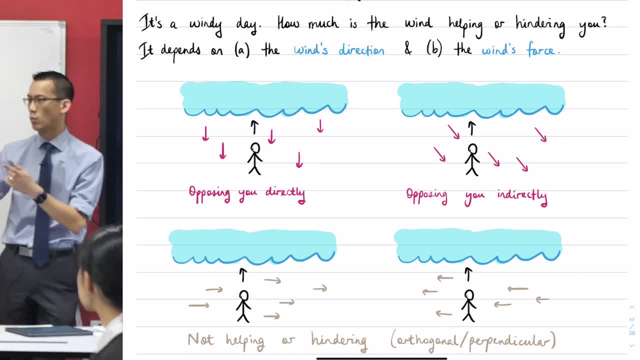 How much the wind is helping or hindering you depends on which way is the wind blowing, what's its direction and how much force is the wind applying, I guess what is its magnitude, right? So in the case where- and this is usually the case, right? 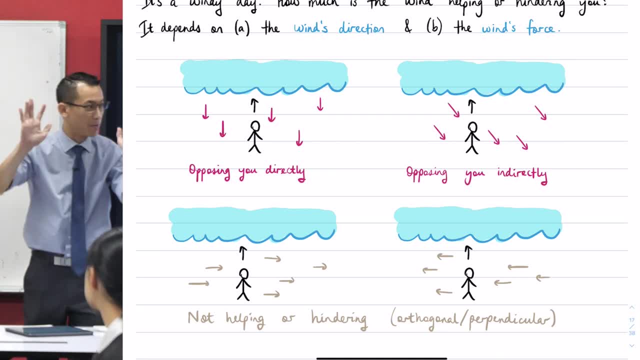 If the water's coming, sorry, the wind is coming out from the ocean and blowing at you, okay, Then it's opposing you Directly, right. If it were coming at an angle, though, right, It's not going to be opposing you as much as if it were, like if you're directly walking into the wind, if you've ever had that experience before, right. 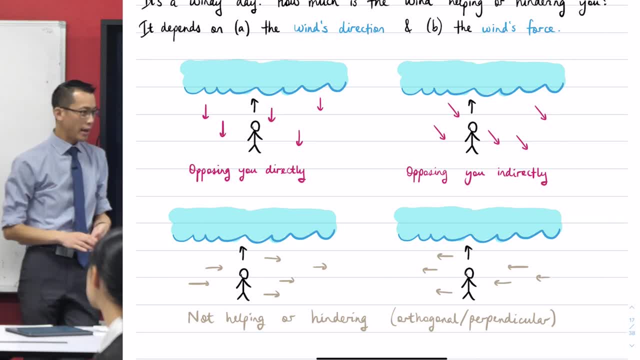 So, in these cases, what is the dot product going to tell you? Well, number one, it's opposing you. so it's going to be negative. when you have this kind of opposing direction of the vectors, And if they're opposing directly, that's the most negative it can get. 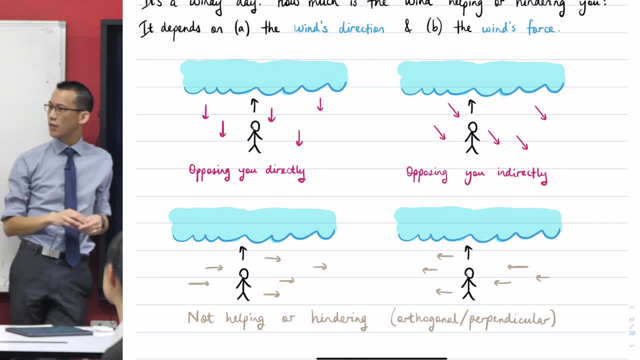 If you're sort of like a little bit negative, like this indirect situation over here, then your dot product is going to be lesser Because the effect on you, the amount it's hindering you from getting to the water, is lesser. 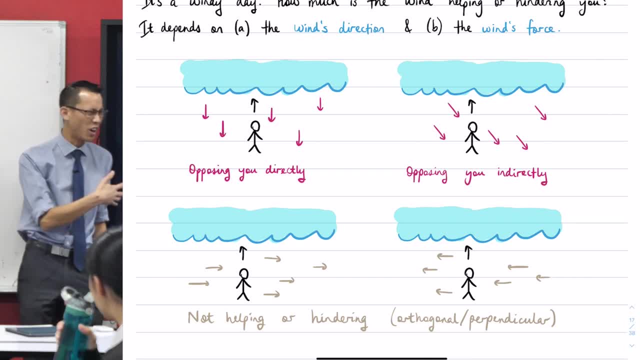 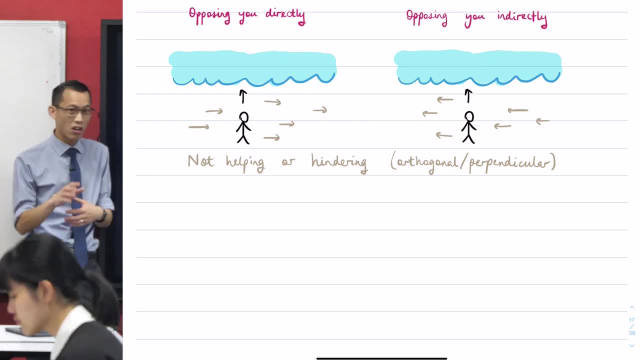 Maybe it'll blow you to a slightly different point in the water than you intended, but you'll still get to the water right Now. if you think about if the wind is just running along the beach, it's going to have an impact on you, but it's not going to slow you down. 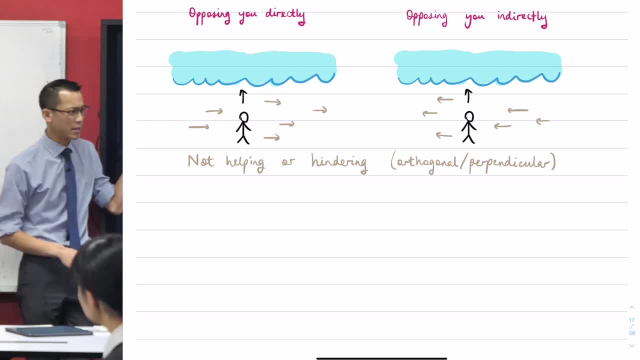 Nor is it going to speed you up in terms of getting to the water. Does that make sense? It's just going to blow you kind of sideways right. You'll still get there if you're still walking at the same pace. And that's why when we say the dot, product of two vectors that are 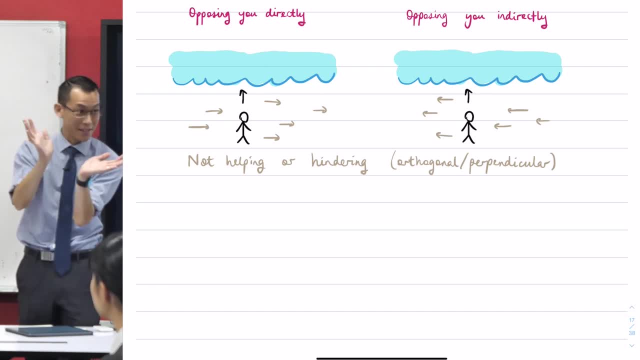 What's that word? again, Now in 2D we can say perpendicular right, But now in three dimensions we would more use the word orthogonal right. So if you've got two orthogonal vectors, like you heading towards the water and then the wind at right angles to you, 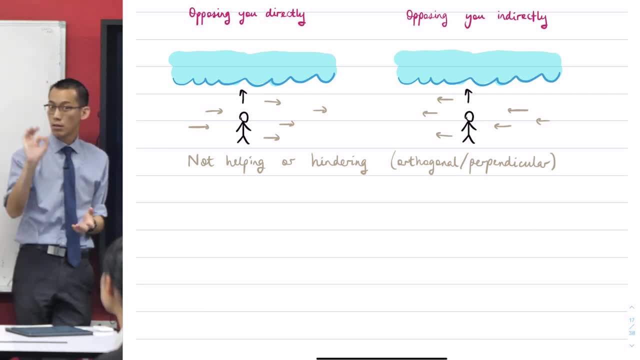 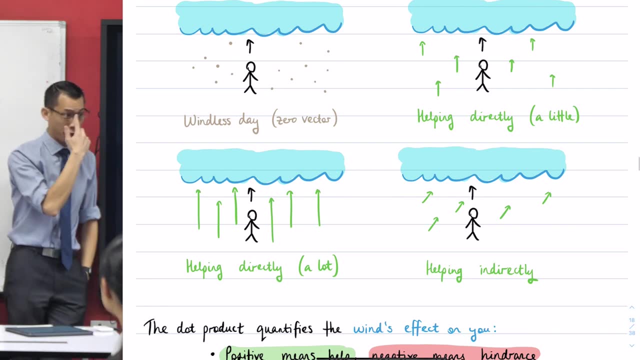 then that gives you a dot product equal to zero right, So they're not really acting on each other at all in terms of trying to get to the water. We know what happens if one of the vectors that you're thinking about is a zero vector. 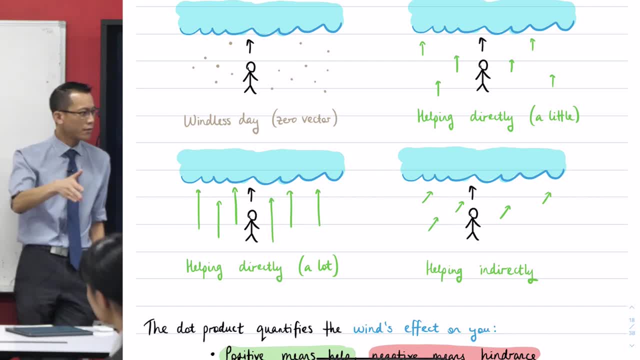 then just by computation, like just doing it in component form, right, Think about multiplying the zeros. you get a dot product of zero as well. Because, again, no impact if there's no wind, right. And then you've got these other situations where the wind is helping you. 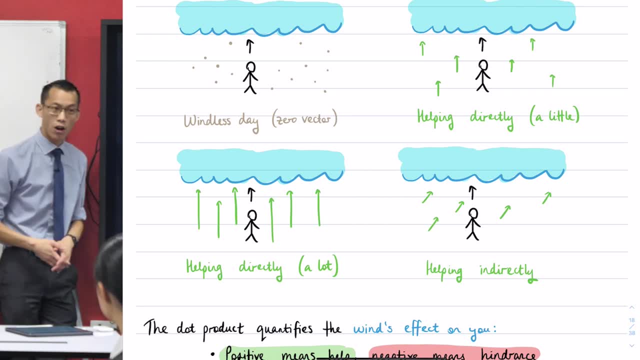 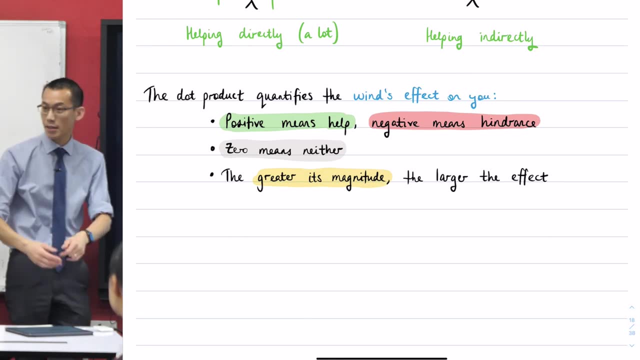 and obviously the more wind there is, the higher that magnitude, the more it helps you out, right? So this is kind of our summary, right? Positive means we're acting in the same direction. Negative means we're acting in opposing directions to some degree. 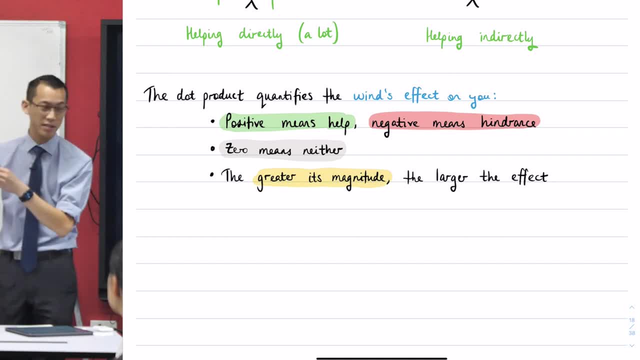 Zero means there's no impact. Right, Mega the actual size, because it's a scalar product. that's the other name, right? So we're going to get a number out at the end. The bigger the magnitude is, the bigger the effect in either direction. 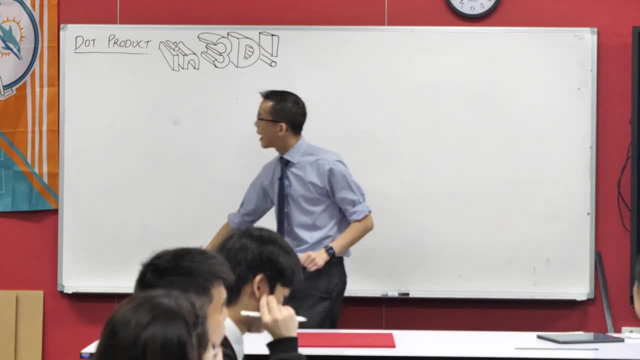 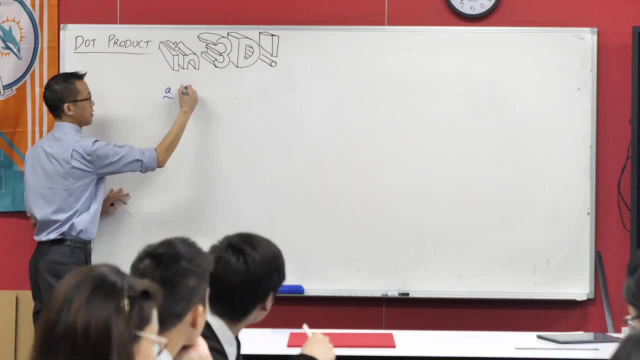 Make sense. Okay, so now let's think about, let's try and come back to this idea of what does that actually mean for the calculation of this thing, If we have pick your pens, if we have two vectors, a and b, and we compute the dot product? 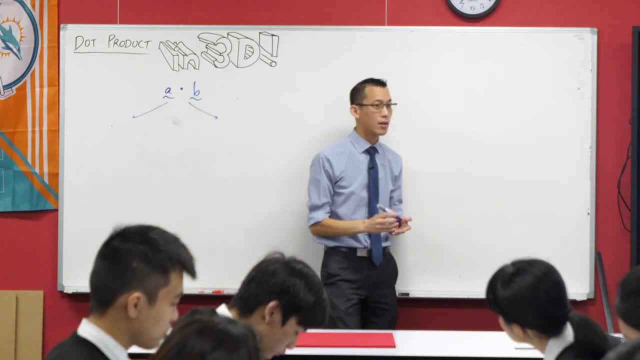 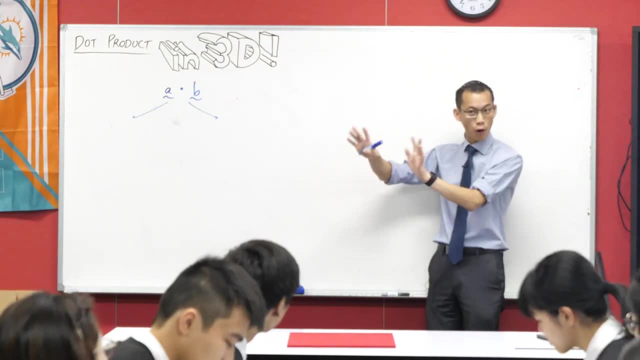 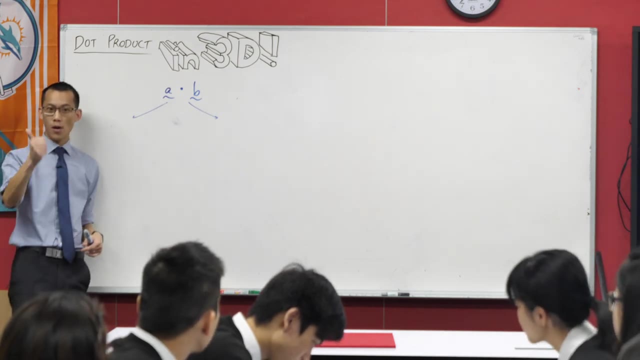 we had two different ways to work out what this thing was, And we did it in two dimensions: firstly by saying component form and then, hopefully you might remember, we used some trigonometry to get to an alternative definition. Now, what I'm going to try and do is go today, number one in 3D, number two in the opposite direction. 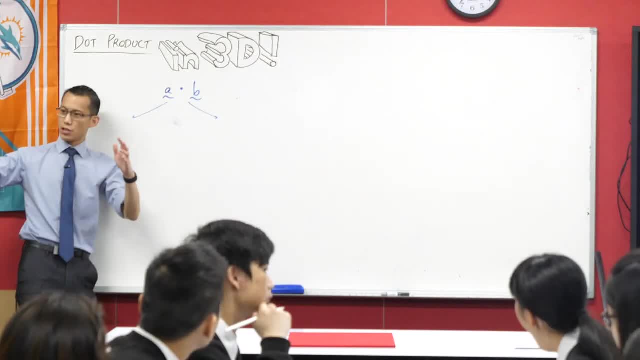 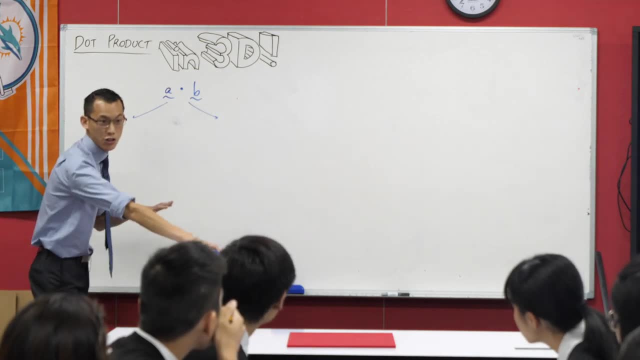 So, based on this idea here of trying to think about, it's to do with magnitude and it's to do with, like, how do the angles of these two vectors relate? Weirdly, I'm going to write down, I'm going to try and visually justify it for you, right? Weirdly, even in 3D. I'm going to try and do it in 3D. Weirdly, even in 3D, I'm going to try and do it in 3D. Weirdly, even in 3D, I'm going to try and do it in 3D. 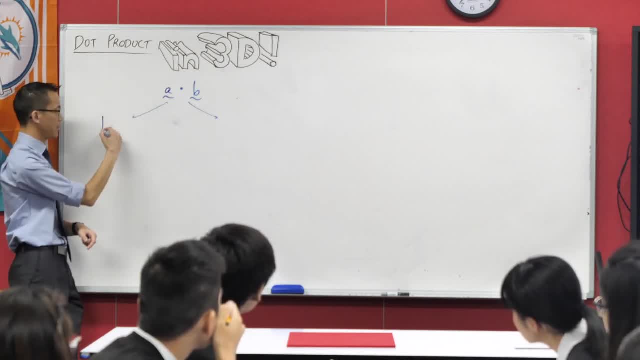 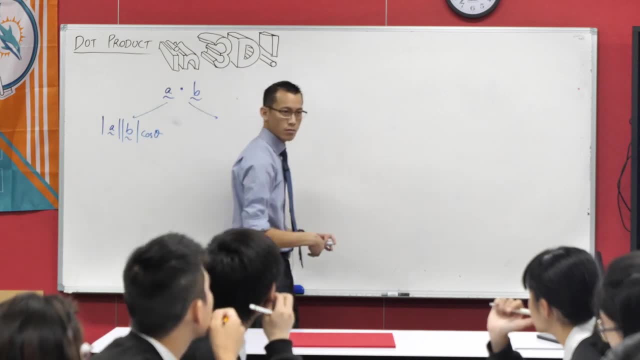 So in two dimensions our dot product for these two things actually has the exact same definition as it does in two dimensions. You remember this formula right? Or maybe you had u's and v's instead of a's and b's? Same diff, right. 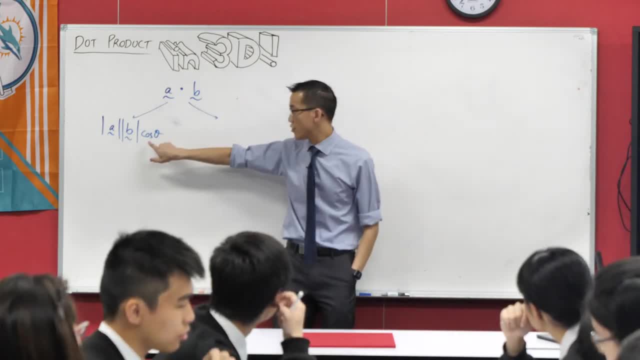 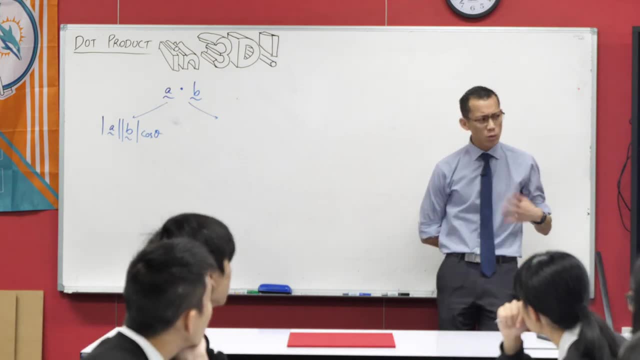 You need to know what the magnitude of the two vectors is, and then you need to consider the angle between them. Now, if you're like me, the first time you see this you're like: how can this be? this seems weird to me that the dot product in 3D looks identical. 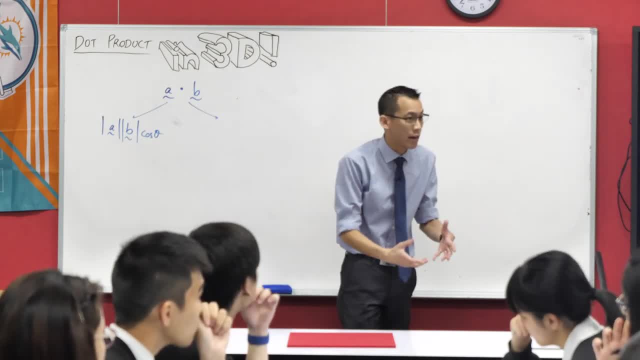 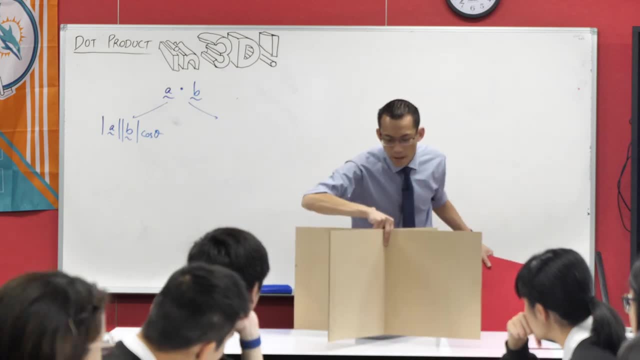 to the dot product in 2D. We're used to it becoming more complicated, right, And I want to try and justify for you why that is not the case. So let me see if I can get an angle. Well, actually, first I'll face it in a more sensible direction. 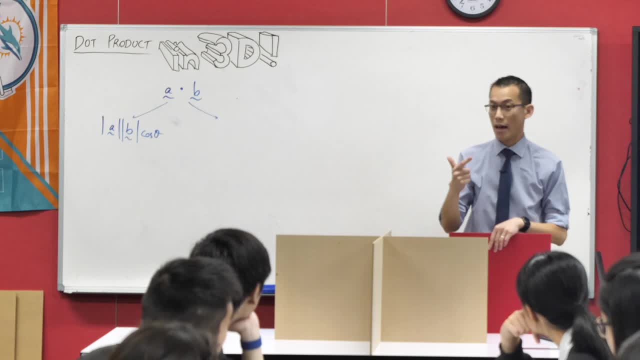 Imagine this as well when we think about our x, y, z coordinate space, right? I want you to imagine these, as I'm going to put it now at an angle so you can see it a little bit better, right? 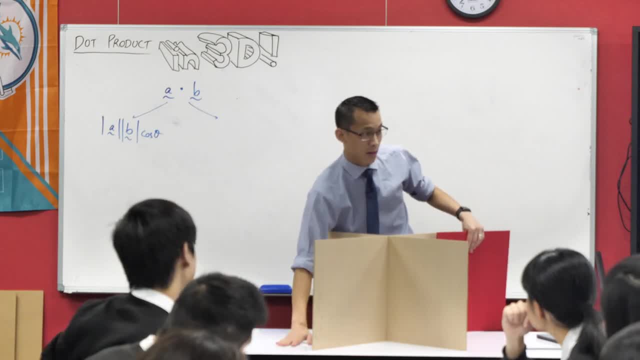 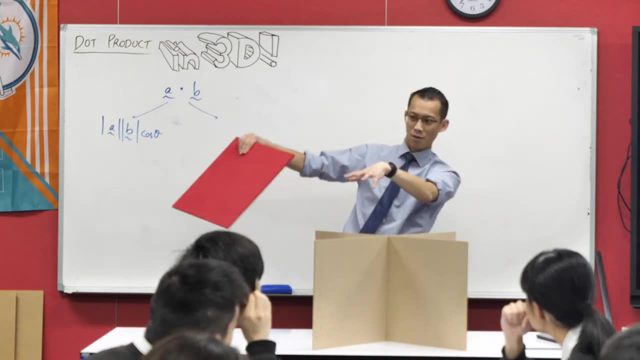 We normally have the x-axis coming out towards you along the ground. we have the y-axis coming off in this direction, usually to your right. okay, And, by the way, please stand up if it's going to help you, because I know there are sort of tall people in the way. 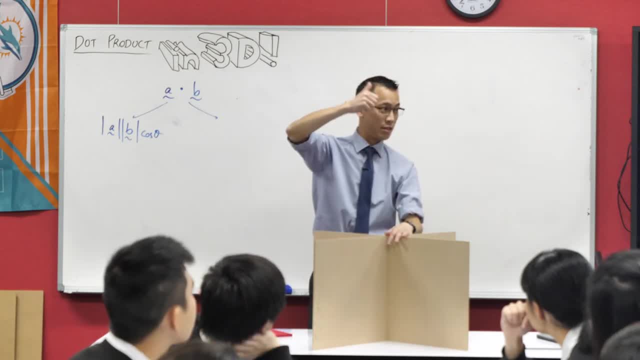 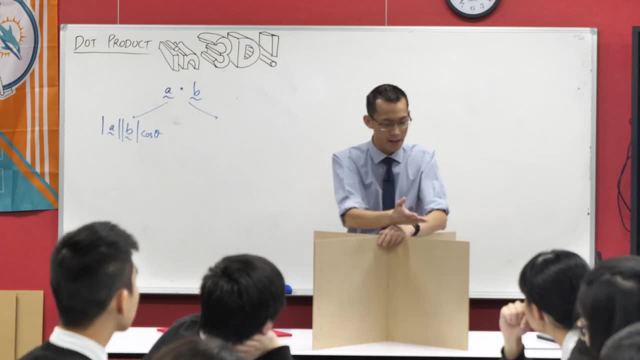 You've got x, y laid flat, and then you've got z coming up into the height, up and down. So far, so good. Now what I want to try and convince you of using this, and you can also do it algebraically, but I find this much more convincing. 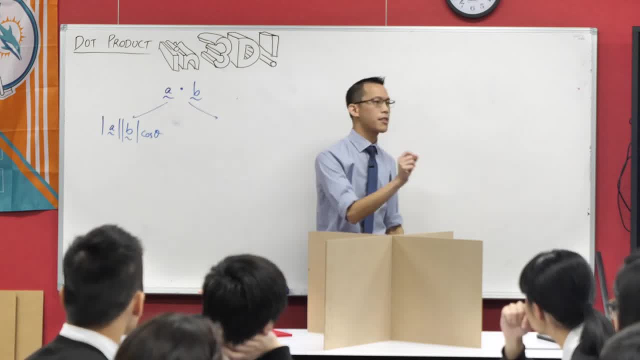 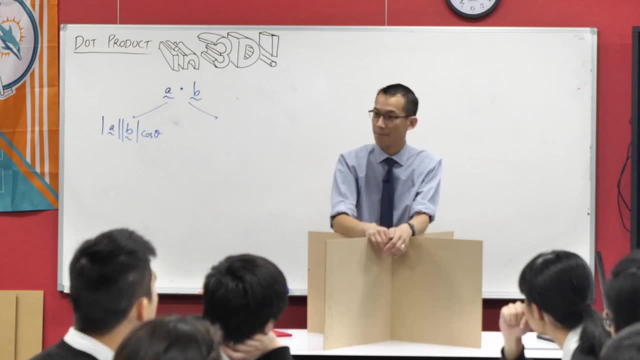 What I want to convince you of is that when you have two vectors in 3D, you can more or less, for the purpose of the for the dot product, consider them in 2D. right, Here's the way I'm going to do it. 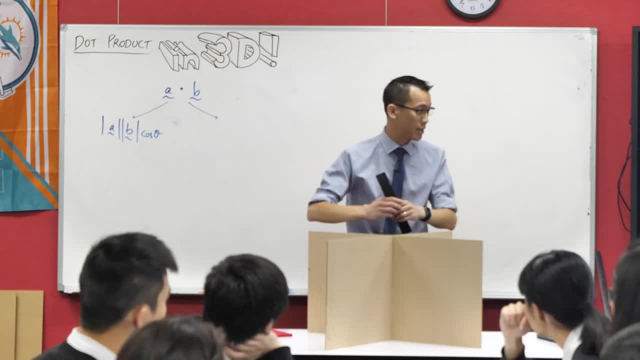 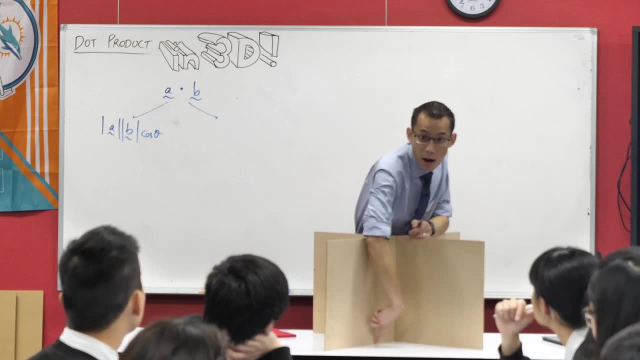 Imagine. imagine you've got two vectors that you're comparing together. Now, for the sake of simplicity and because of the fact that I only have two hands, let's just treat the positive part of the x-axis that's coming out at you. 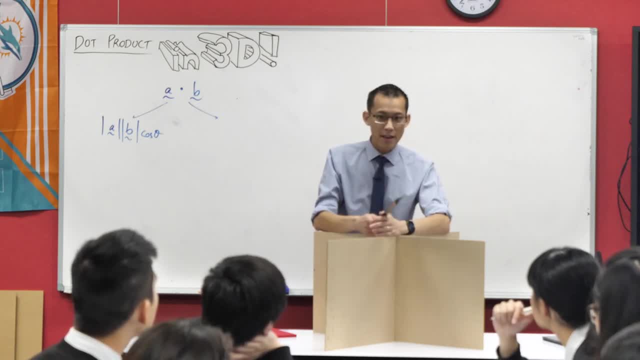 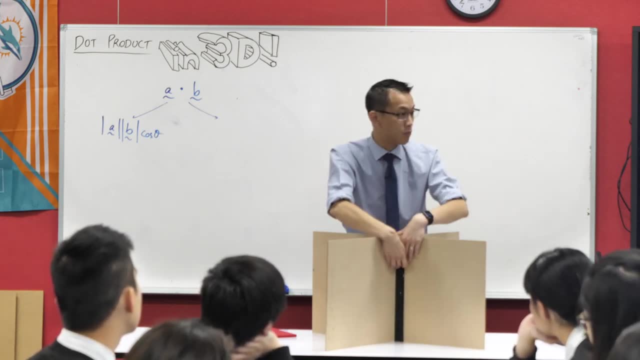 let's just treat that as one of our two vectors, okay. And then the other vector is going to be this black one. right Now, imagine I'm going to do this for simplicity's sake first, right. Imagine, if I make it. well, just the z-axis. 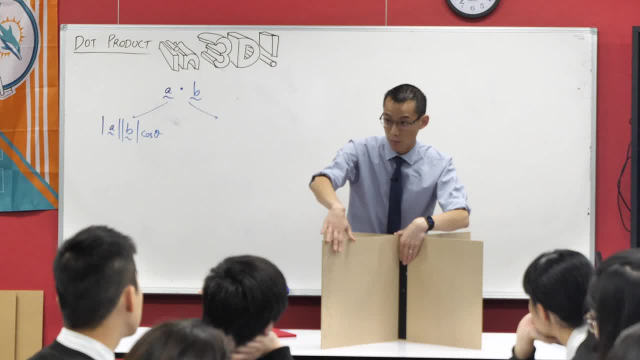 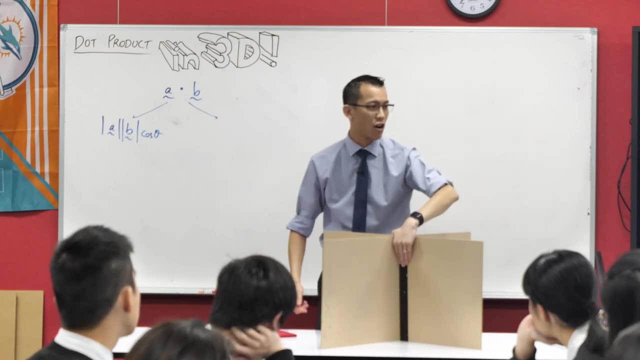 Right. Do you see that Now, literally by definition, you can see these pieces of wood here that help you out. You can obviously see that that first vector and my second vector- they clearly share a plane. Does that make sense? 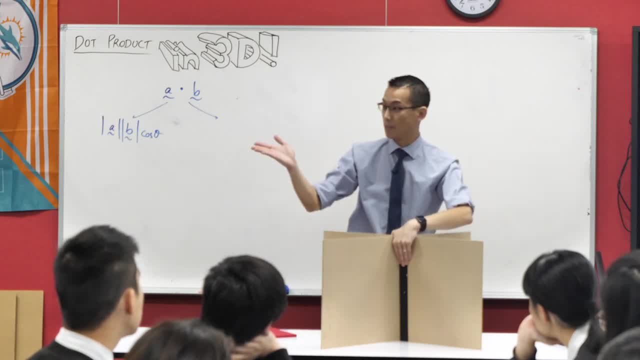 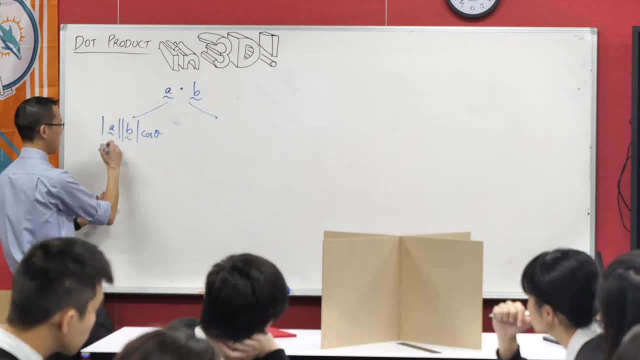 I mean, in this case it's the xz plane. So the fancy word for this- and I should write this down, and so should you, the fancy word for this- is that they are coplanar- Coplanar. Do you remember when we talked about points being collinear? 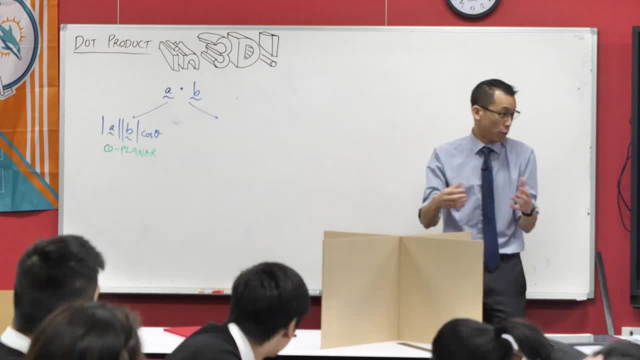 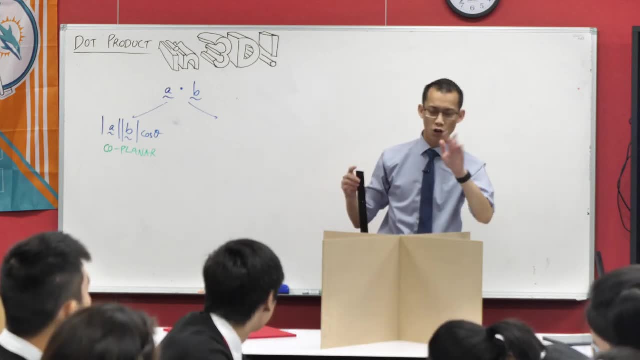 Collinear means points on a plane. Collinear means points on the same line. Coplanar means you've got two vectors and they're on the same plane. No big deal, Okay. So if I had a simple situation like this: x-axis, z-axis. 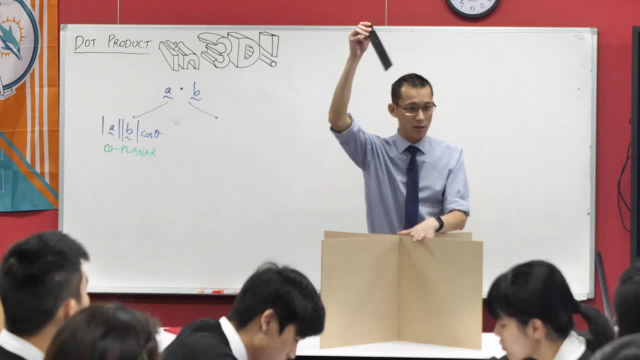 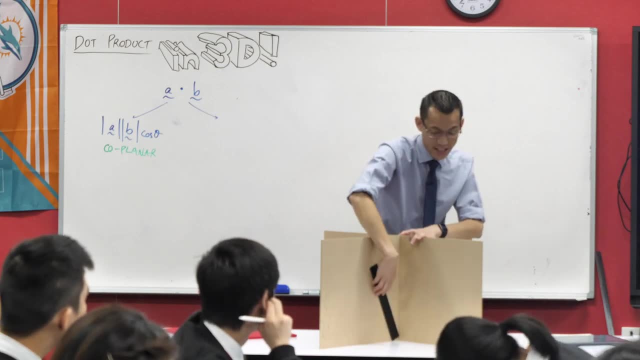 of course they share a plane. Once you've written that down, look up again and have a look at what I'm about to do to this black vector right. Obviously, I can rotate it around along the xz plane right, And it's still on this same 2D space. 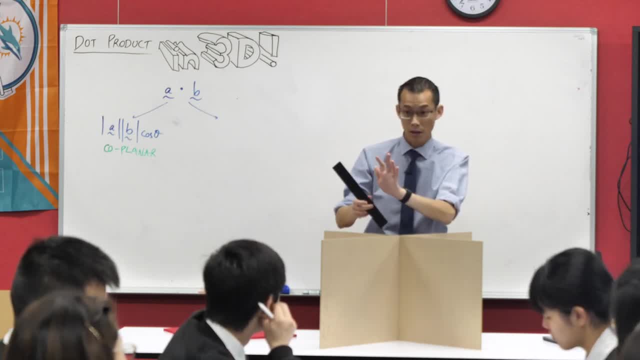 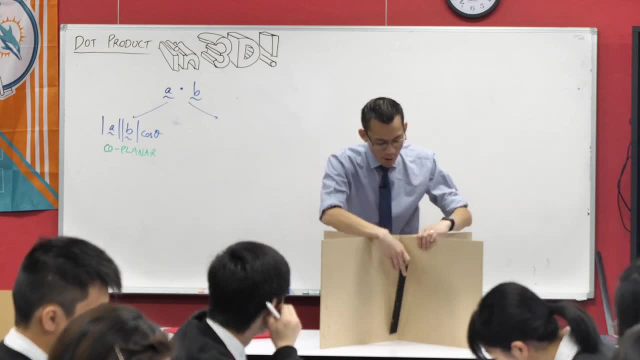 I can do this kind of rotation to it and it stays on the same plane, Agreed. So I haven't like. even though I have this degree of freedom, I'm still going to be coplanar, okay. But now imagine what happens if I try and come off the xz plane. okay, 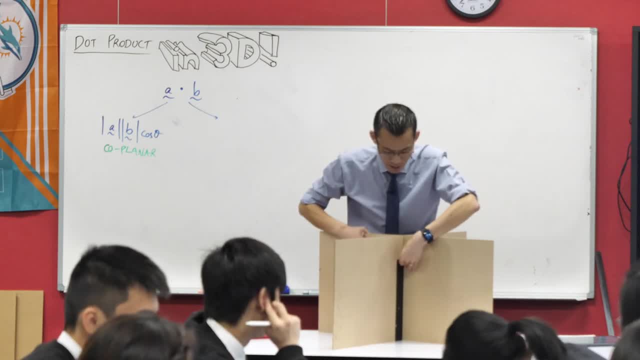 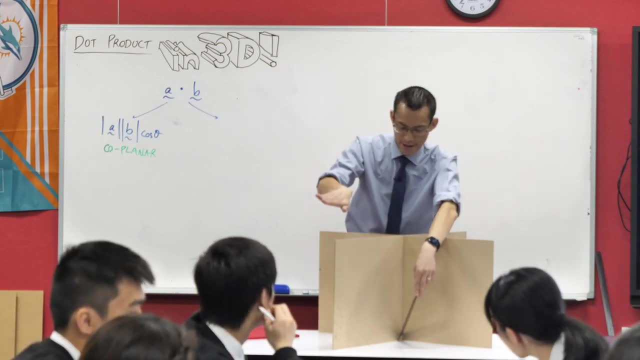 So I'm going to start again with this simple situation: z-axis. Now, let's like put it over here, right? So it's coming out sort of diagonal into the first octant, is what we called it before, because x and y and z are all positive, okay. 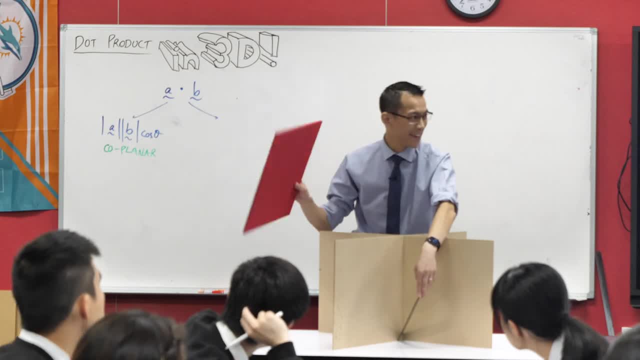 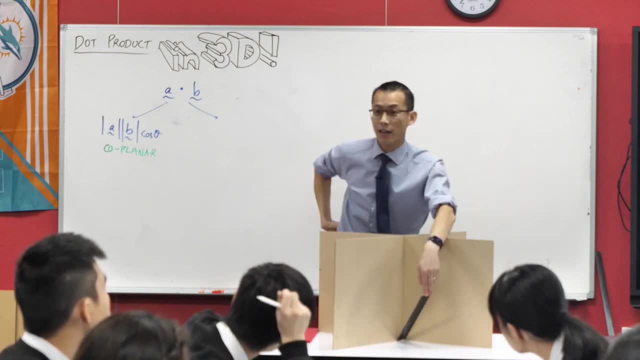 Can you see? can you yet visualize? I'm going to help you in a second, don't worry. but can you visualize the plane that is shared by the x-axis and my second vector? Can you visualize it right Now? what I would do, what I think is the easiest way to think about it, is: 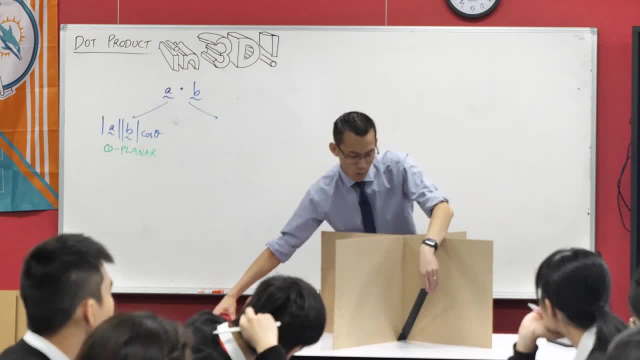 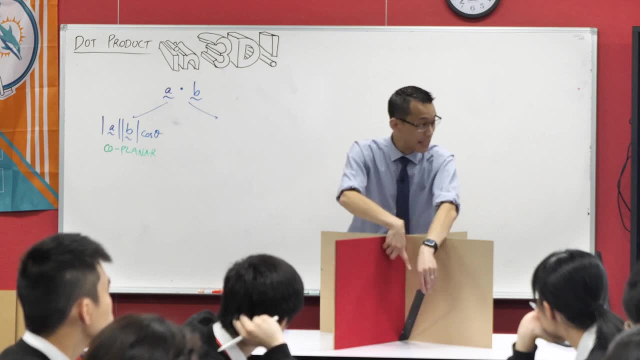 start from the xz plane that we were on before right, And then think about what would happen if, like how far do you have to rotate this xz plane and in which direction do you have to rotate it to get to my second vector?